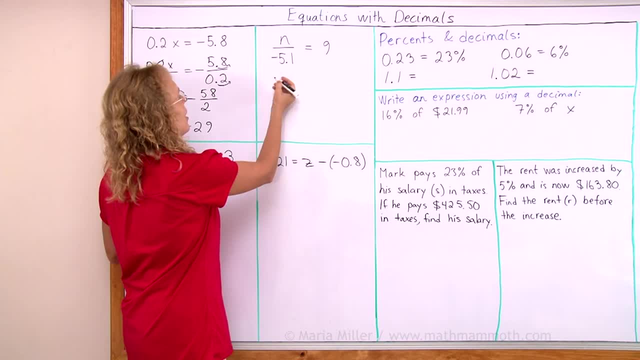 multiplying both sides by this number. Okay, So we multiply negative 5.1 times this, n over 5.1. And then on this side the same thing: Negative 5.1 times 9.. Okay, And here of course this now cancels, so we get n alone, which is what we want, And it's now isolated, And here 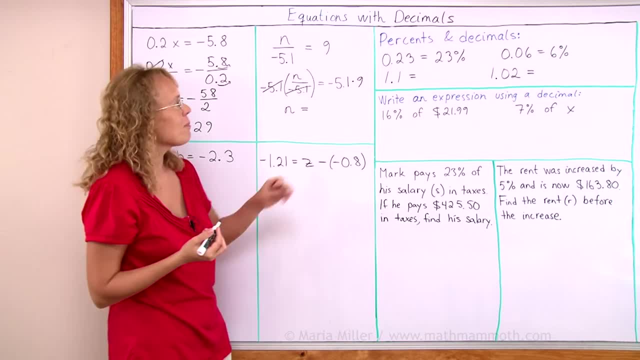 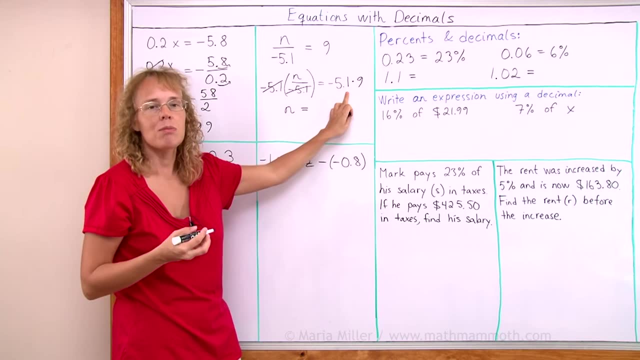 we need to multiply this. We can do the multiplication mentally, because we just multiply 9 times 5. 45. And then 9 times one tenth, Which is 9 tenths. So we get 45 and 9 tenths, but it 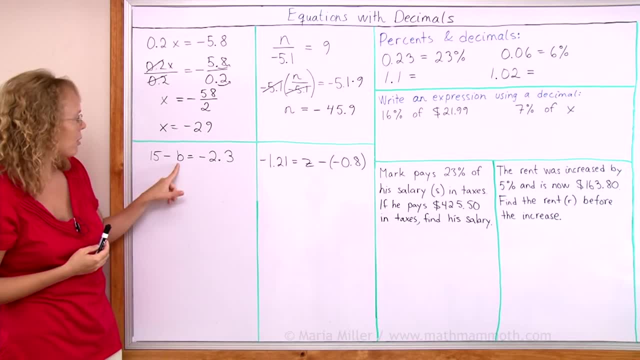 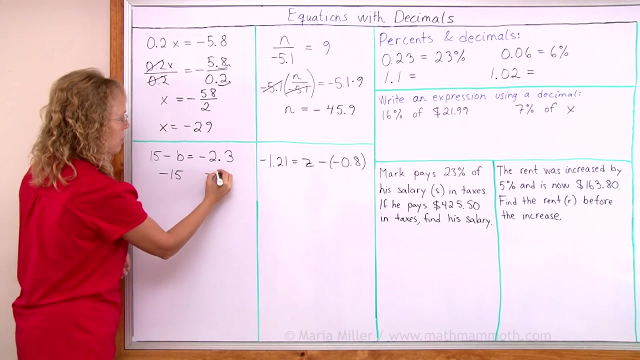 is negative. Here we have the variable here as a negative, Negative b Or minus b, And then there's 15. here 15 is added. So to isolate negative b here, then I would subtract 15 from both sides, So we get- Let me write it here- Subtract 15.. Subtract 15 from both sides, And here: 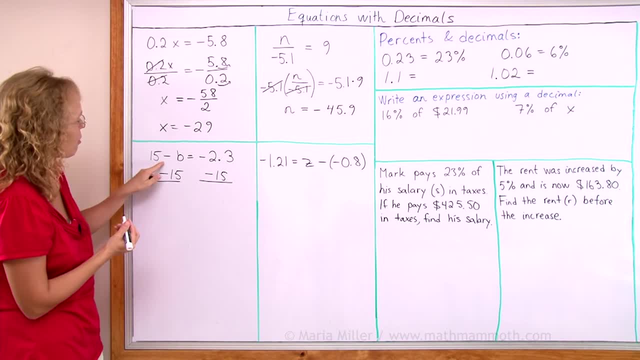 15 minus 15 of course leaves zero, Nothing. So we are left with this negative b. On this side I have negative 15 and then negative 2.3. Lots of negatives. So I add the absolute values, Right, I add 15 and 2.3. That's 17.3. 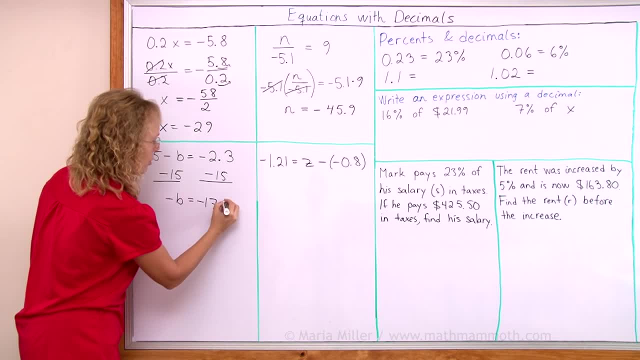 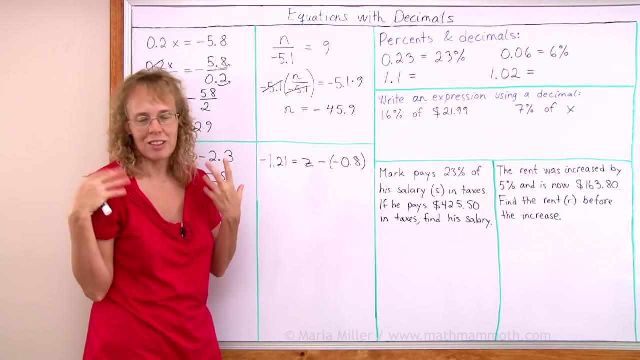 but the whole thing is negative. So I get 17.. Negative 17.3.. And of course, if opposite of b equals this negative number, then b must equal 17.3.. Here, Here, Here I will simplify first, because this double negative is always a little complicated to. 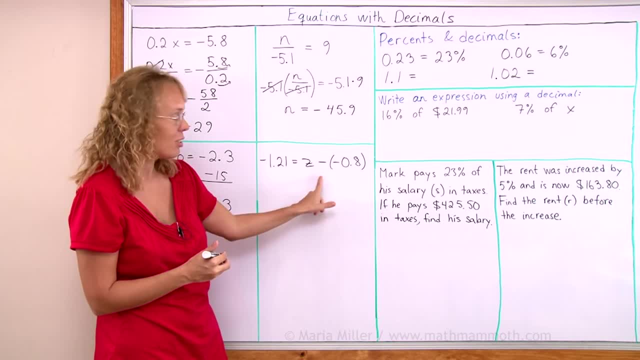 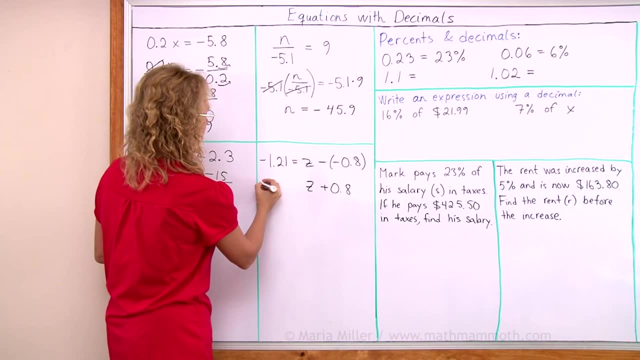 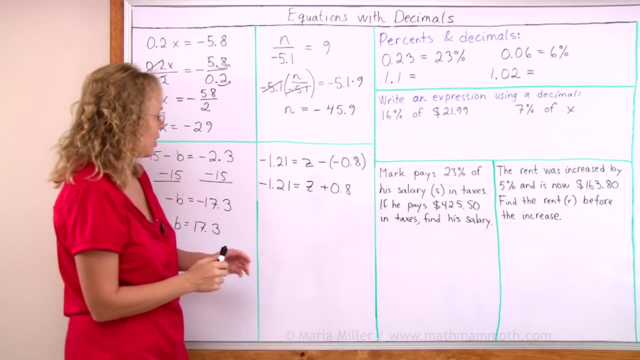 handle otherwise. But it becomes very simple when I change it to just a plus Right, So I will rewrite this as z plus 0.8.. On this side it's negative 1.21.. And now, if you want to, you can flip these two sides so that you get your variable on the left side, as is customary. 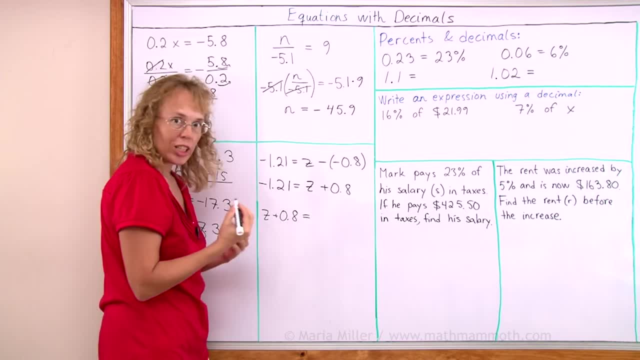 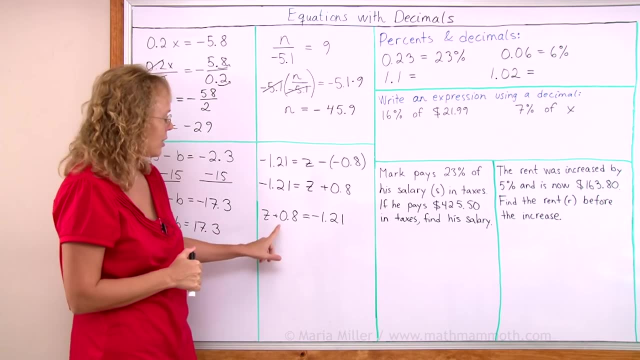 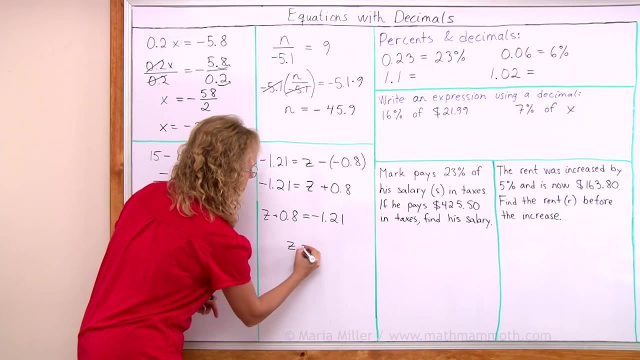 It's not absolutely necessary, but it often makes sense, But it often makes things look easier. Okay, And now? it is a simple addition equation. So we just subtract from both sides this number. So I subtract 8 tenths. It leaves z alone here. 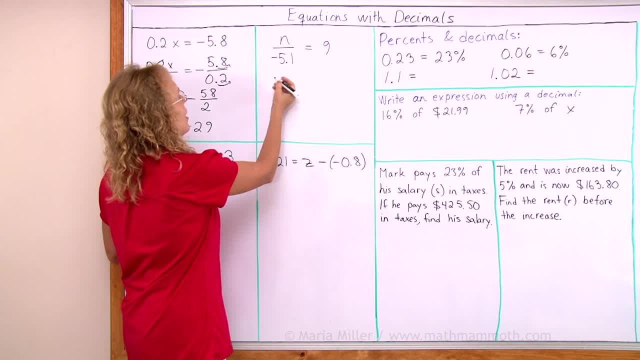 multiplying both sides by this number. Okay, So we multiply negative 5.1 times this, n over 5.1. And then on this side the same thing: Negative 5.1 times 9.. Okay, And here of course these now cancel, so we get n alone, which is what we want, And it's now isolated And here 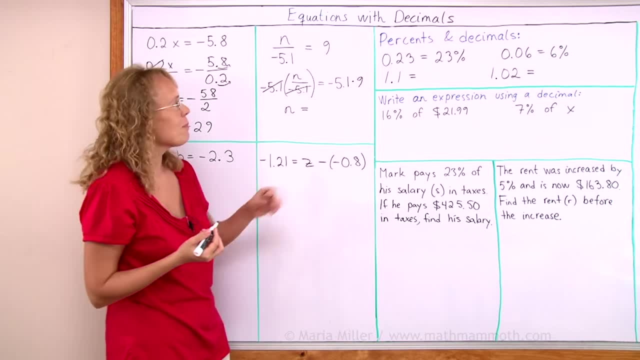 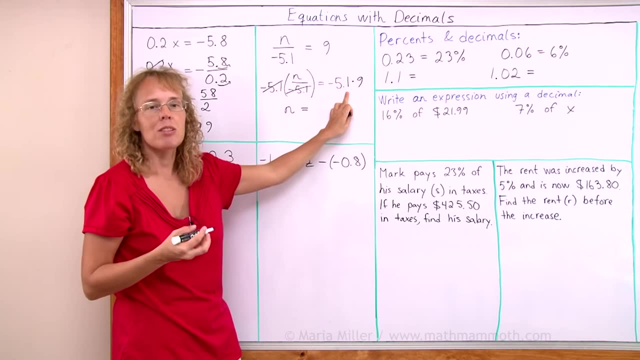 we need to multiply this. We can do the multiplication mentally, because we just multiply 9 times 5.. 45. And then 9 times 1 tenth, which is 9 tenths. So we get 45 and 9 tenths, but it is. 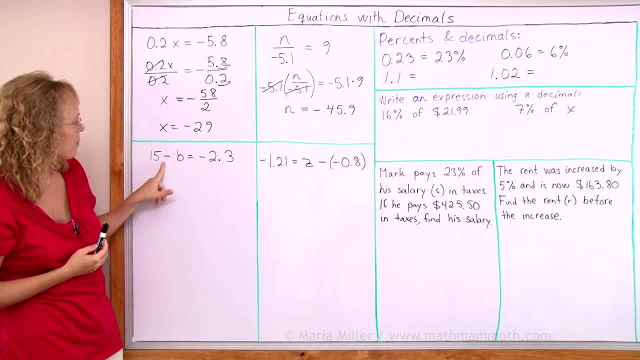 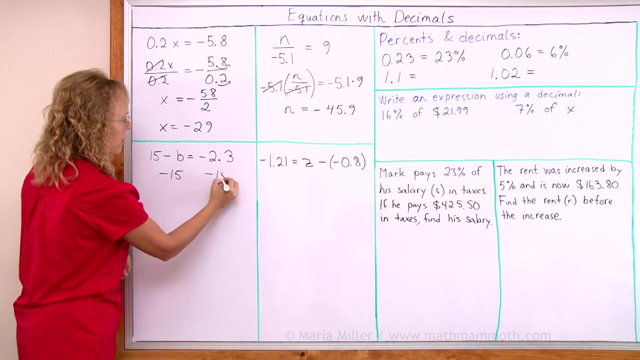 negative. Here we have the variable here as a negative, Negative b or minus b, And then there's 15. here 15 is added. So to isolate negative b here, then I would subtract 15 from both sides, So we get- let me write it here- Subtract 15.. Subtract 15 from both sides, And here: 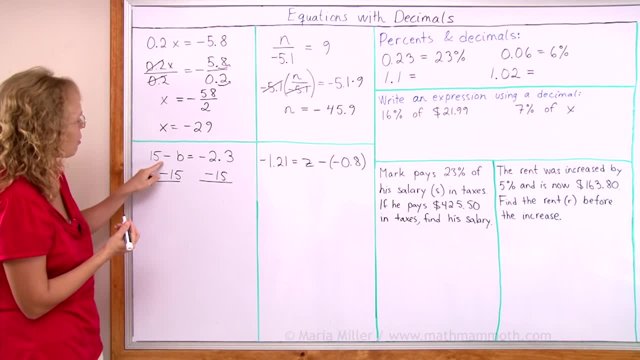 15 minus 15 of course leaves 0. So we are left with this negative b. On this side I have negative 15 and then negative 2.3. Lots of negatives. So I add the absolute values, Right, I add 15 and 2.3. That's 17.3. 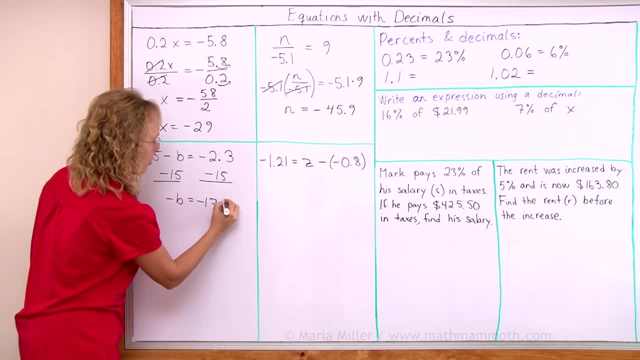 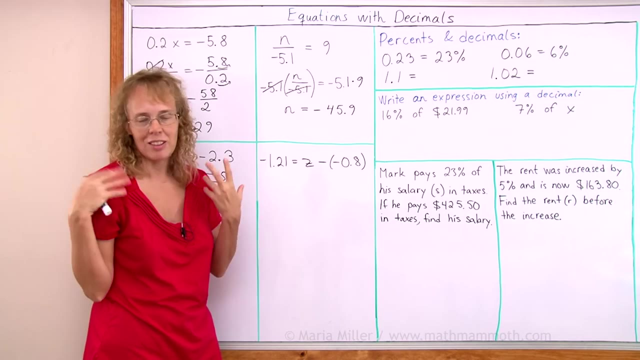 but the whole thing is negative. So I get 17, negative 17.3. And of course, if opposite of b equals this negative number, then b must equal 17.3.. Here I will simplify first, because this double negative is always a little complicated to. 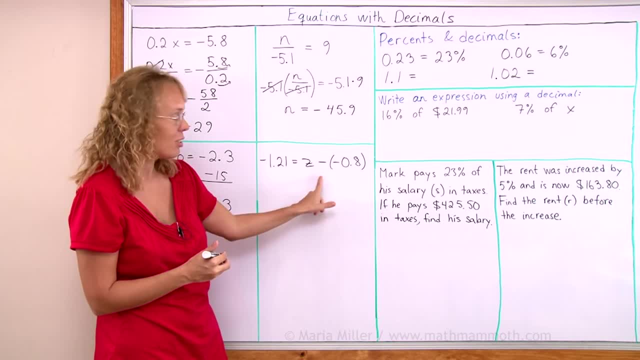 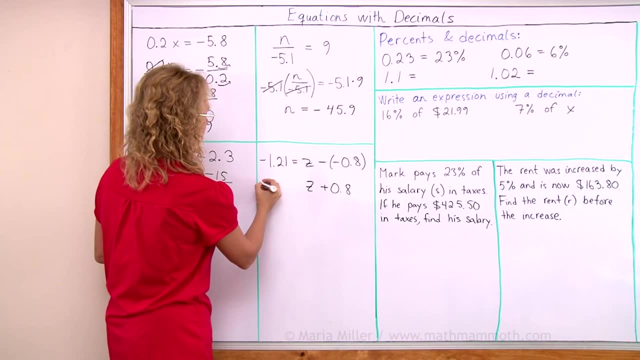 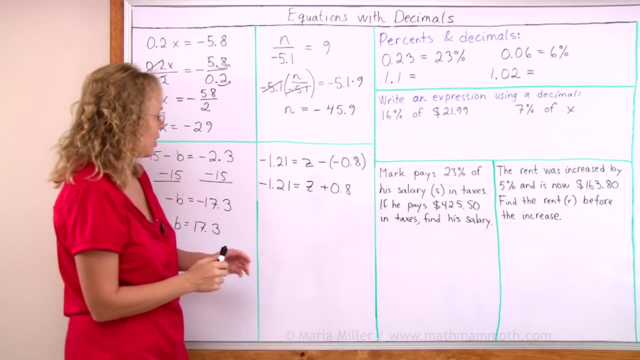 handle otherwise. but it becomes very simple when I change it to just a plus Right, So I will rewrite this as z plus 0.8.. On this side it's negative 1.21.. And now, if you want to, you can flip these two sides so that you get your variable on the left side, as is customary. 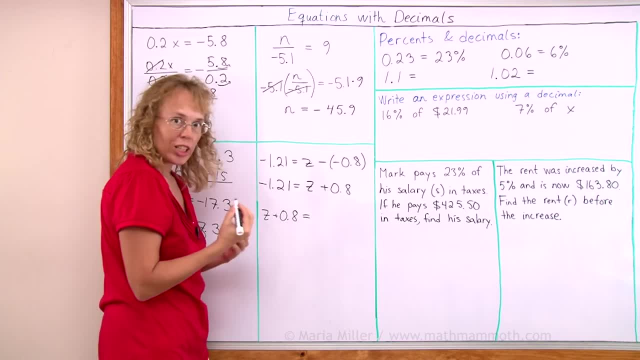 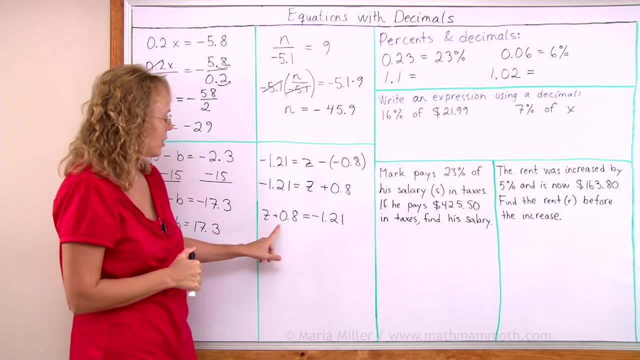 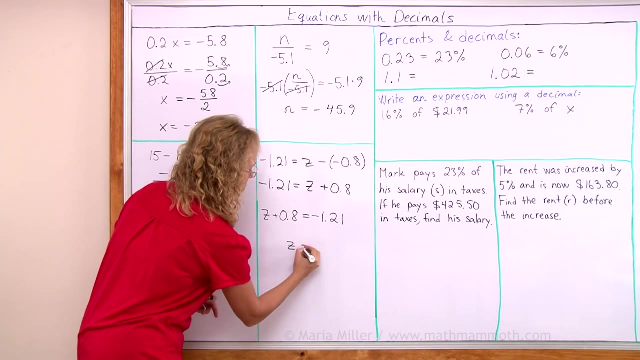 It's not absolutely necessary, but it often makes sense. It often makes things look easier. Okay, And now? it is a simple addition equation. so we just subtract from both sides this number. So I subtract 8 tenths. it leaves z alone here.